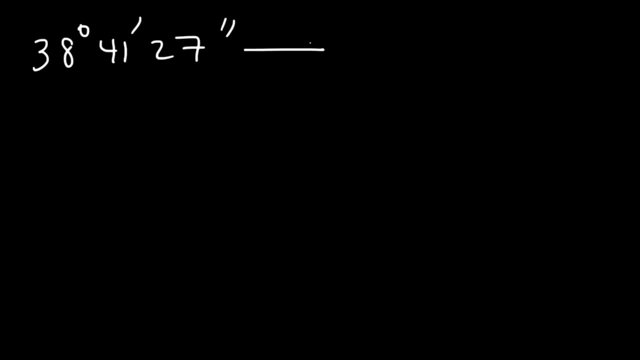 and 27 seconds into a decimal in degrees, Round your answer to four decimal places. So this is equal to 38 plus 41 over 60 plus 27, divided by 3,600.. And type this in exactly the way you see it. 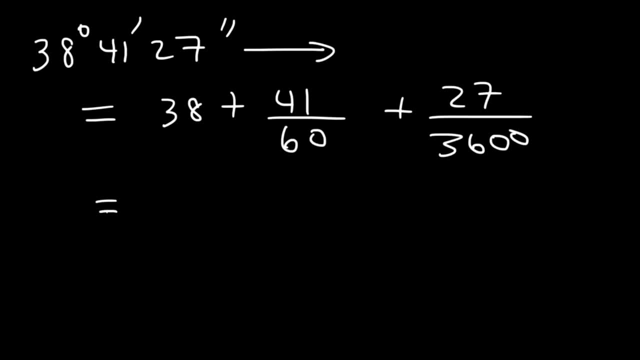 in your calculator. So the answer is 38.. 38.6908 degrees. Now let's try one more example. Try this one: 53 degrees, 18 minutes and 39 seconds. Go ahead and convert that to a decimal in degrees, So it's just going to be 53 plus 18 divided. 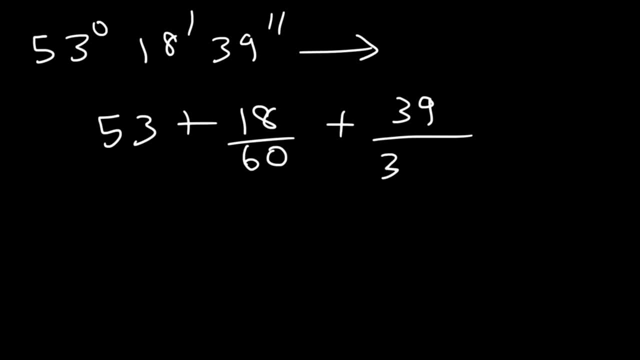 by 60 plus 39 divided by 3,600. And that's going to be about 53.3108 degrees. So now you know how to convert DMS to a decimal in degrees. Now let's convert a decimal in degrees back into DMS, that is, degrees minutes. 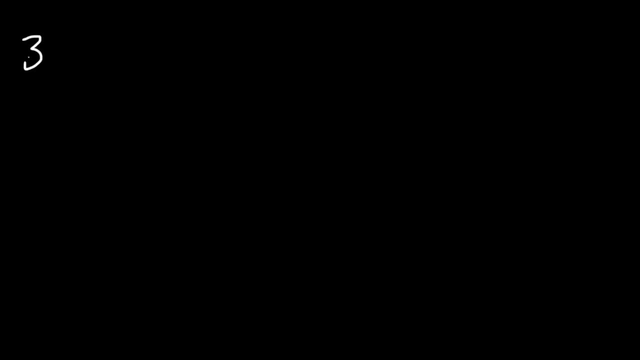 and seconds. So let's say, if we have a value value 38 degrees, actually 38.4256 degrees, Let's convert that to degrees, minutes and seconds. So how can we do this? So the whole number that you see here, 38, that's your. 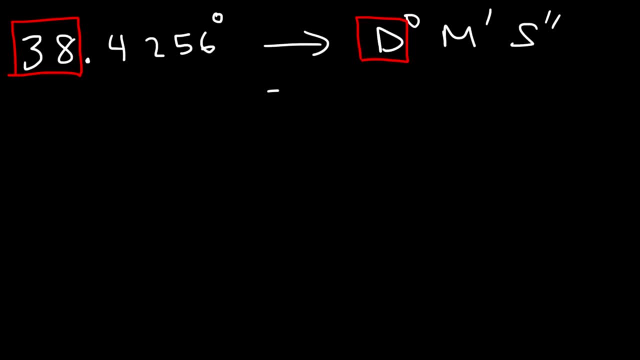 value in degrees. So what we have so far is 38 degrees. Now take the decimal value 0.4256, and what you want to do is you want to multiply that by 60.. 0.4256 times 60,, that's 25.536.. 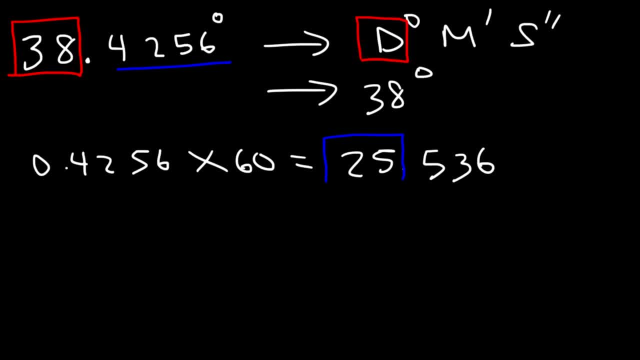 Now take the whole number 25, and write that as your value for minutes. So it's 25 minutes. Now take the decimal that remains, which is 0.536, and multiply that by 60.. 0.536 times 60 is 32.16.. Now you want to round. 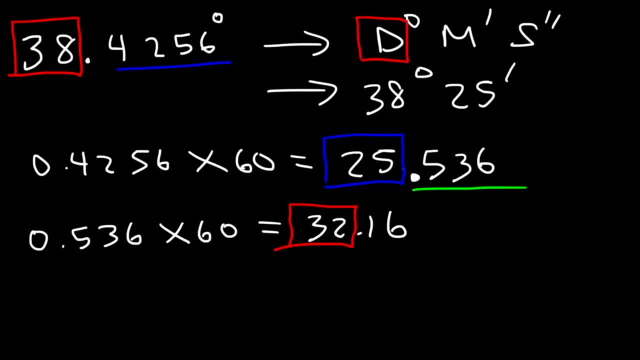 this to your nearest whole number. So in this case that's 32.. And so that's going to be the number of seconds. So we have 32 seconds. So this is our answer: 38 degrees, 25 minutes and 32 seconds. Now, to confirm the answer, type this in your calculator: 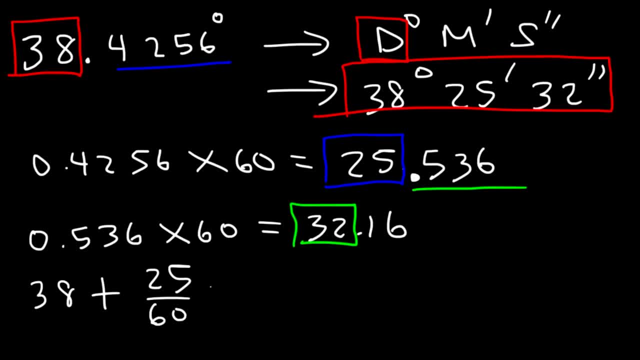 38 plus 25 divided by 60, plus 32 divided by 3600.. It should give us our original value. Now the answer won't be exact, but it's going to be close to it. What I have is 38.4255. 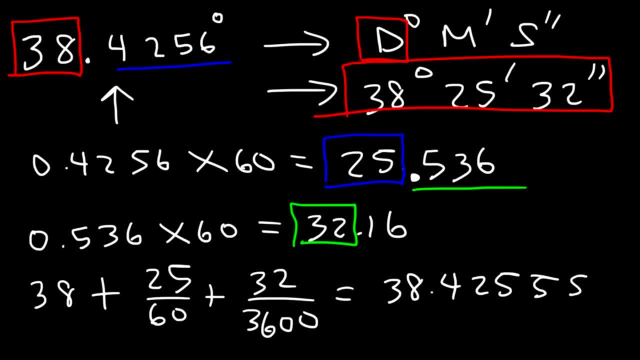 repeated. So instead of writing 55 repeated, if you round it this is going to be five six. The reason why is that it's not going to be an exact answer is because we didn't use the 16, we use. The answer is 32.16 to 32.. So this answer is going to be very close to the answer. 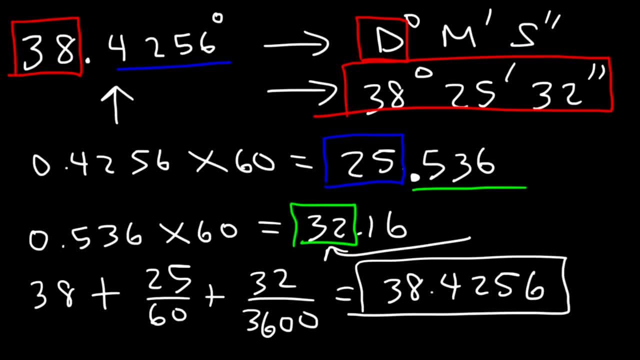 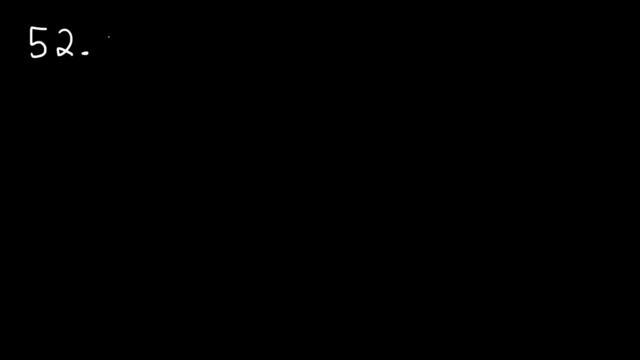 dużo más� rooted una dubios no LIKE. we ronde conmeye answer that you started with in the beginning, and if it's very, very close, then you know you did it correctly. now let's try some other examples. let's say, if we have 52.3, 175 degrees, convert that to DMS degrees, minutes and seconds. so 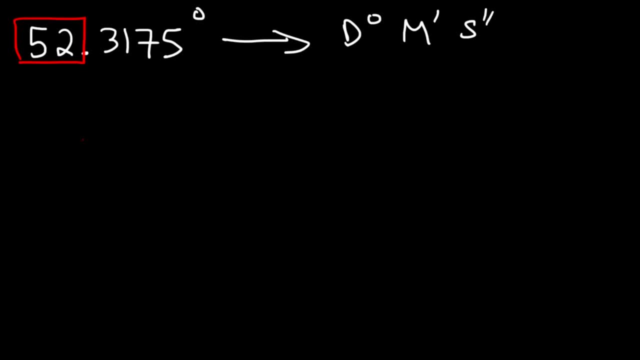 first, we can see that it's going to be 52 degrees. that's the first number that we need to write. now let's take the decimal value, point 3175, and let's multiply it by 60, so this is going to be 19.05 and the number 19 that's how many. 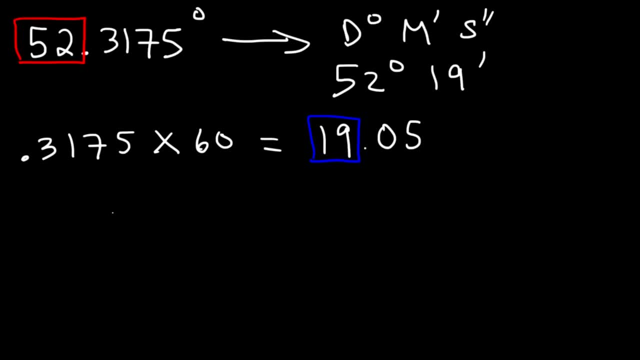 minutes that we have now. let's take the remaining value, point 05, and let's multiply the remaining value, point 05, and let's multiply that by 60. point 05 times 60 is 3 and that's it, an exact answer. so this is. 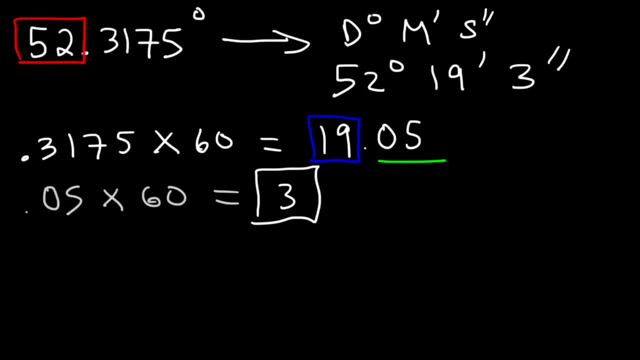 going to be 3 seconds now. let's confirm the answer. so type this in your calculator: 52 plus 19 divided by 60 plus 3 divided by 3600. you should always do a quick check to see if you have the right answer and you. 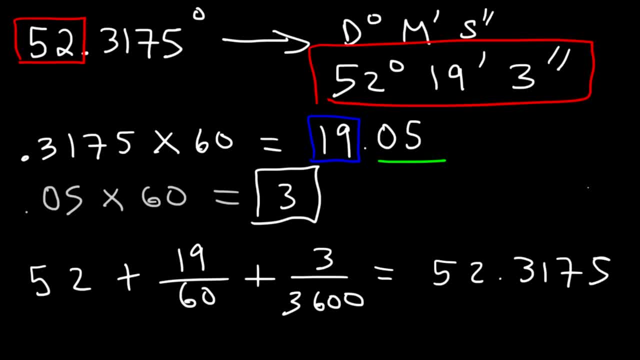 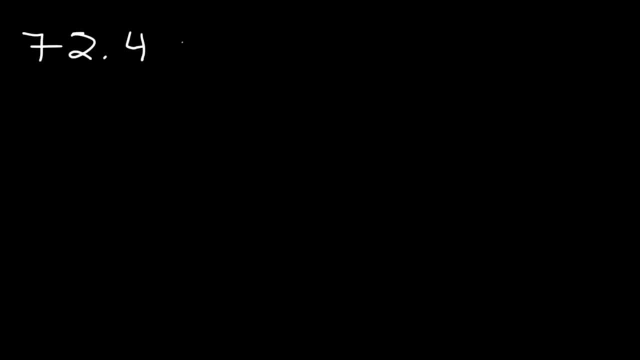 do indeed get 52.3, 175, so we know that this answer is correct. let's try one more example: 72.4, 813 degrees. go ahead and pause the video and convert it to degrees, minutes, seconds. so let's write the first number, 72. so we have 72 degrees. now let's take the. 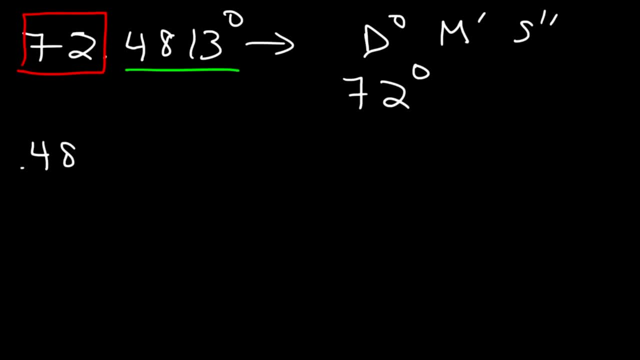 decimal value point 4813, and let's multiply that by 60, so this is going to be 28.878, and so let's record this number, so we have 28 minutes. and then let's take the decimal value point 878 and let's 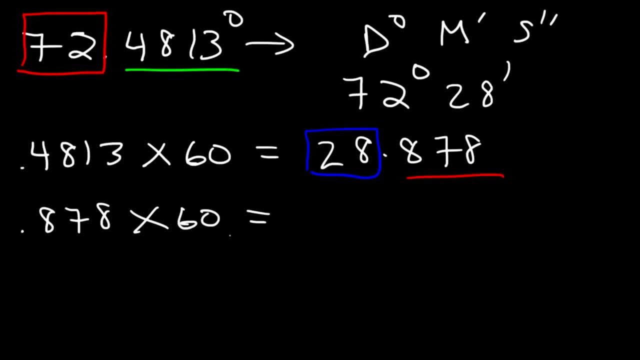 multiply that by 60. point 878 times 60, that's 52.68. now what you want to do is you want to round this number six. we need to because of the six. we need to round the two, two or three. so we got around up. so instead of rounding, 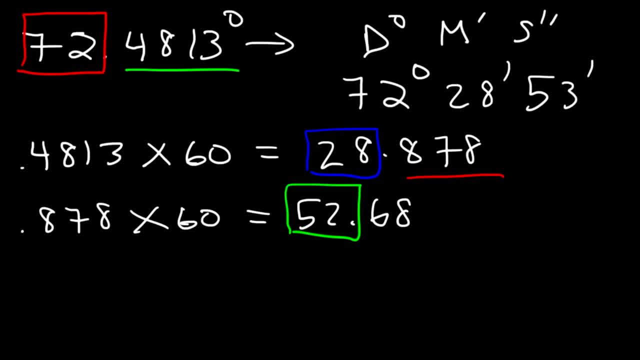 into 52, we're going to run into 53 and that's the answer. now, because we rounded it, this answer is not exact when converting this back to this number, but it should be close. so if we type in 72 plus 28 divided by 60 plus 53 divided by: 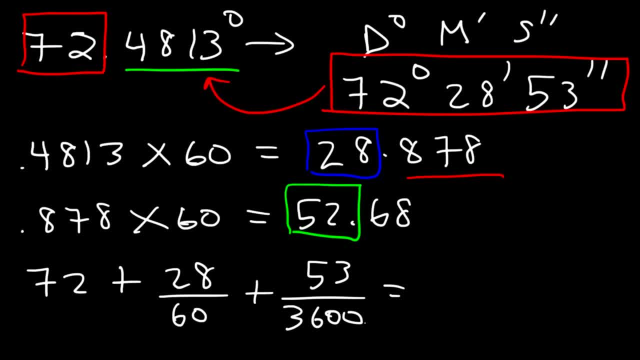 3600, we're going to get 72.4814 if you run it. if you don't run it, it's like 139. now let's see what would happen if we kept it as 52. if we kept it at 52, it would be 72.4814. 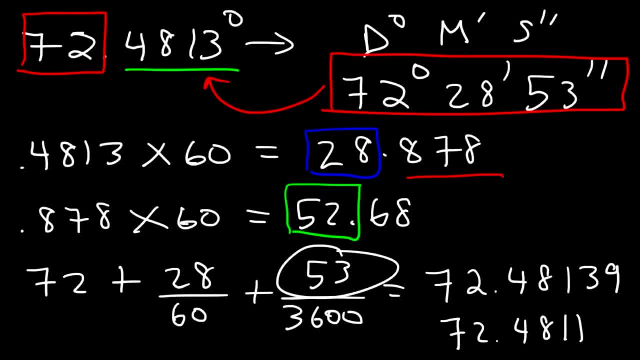 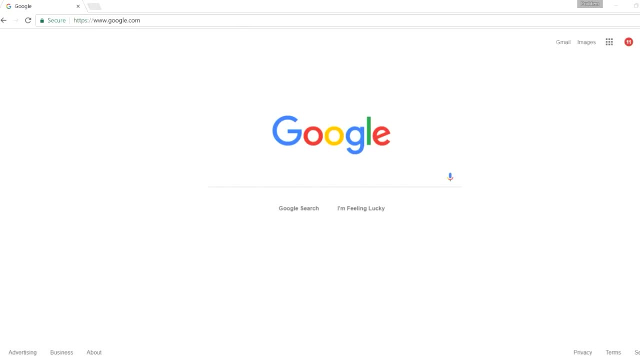 which is further than 14. so this is closer to the actual answer. so, therefore, this is our best estimation and that's the answer for this problem. now for those of you who want access to my complete online trigonometry course, here's where you can find it: go to udemycom and then in the search box. 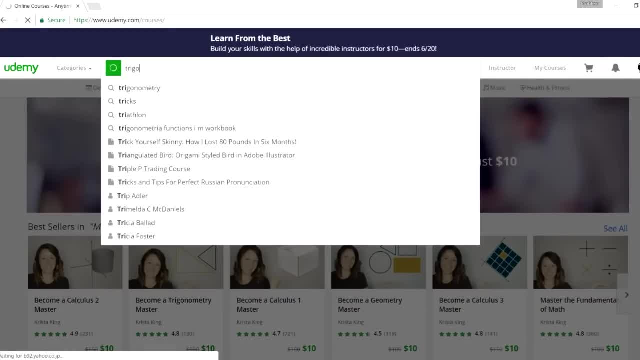 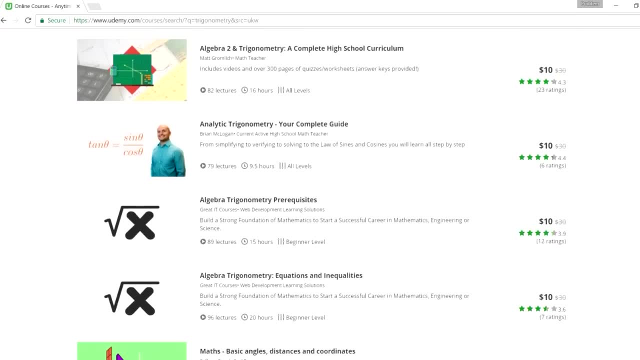 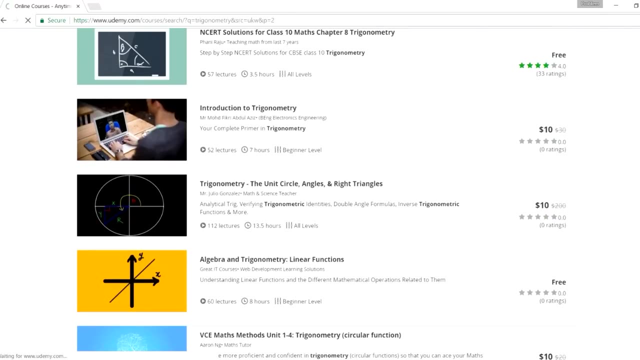 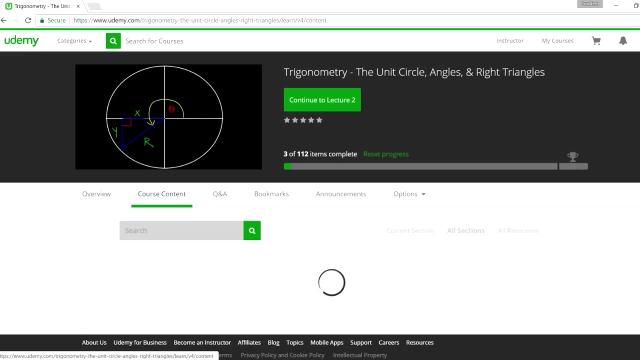 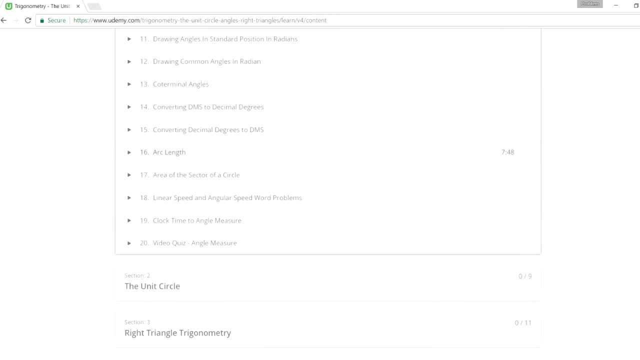 you can just search for trigonometry and you can see. my course is basically the one with the black background, and then here is it. I'm still adding more lectures, but here's what I have so far. introduction to angles: drawn angles. converting degrees into radians. linear speed, angler speed. 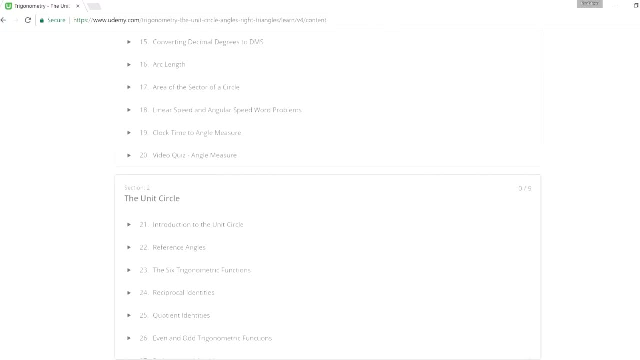 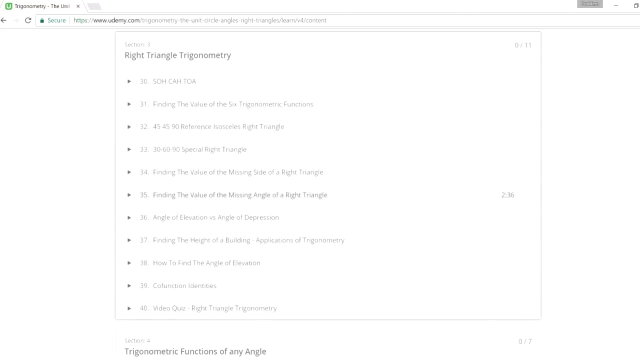 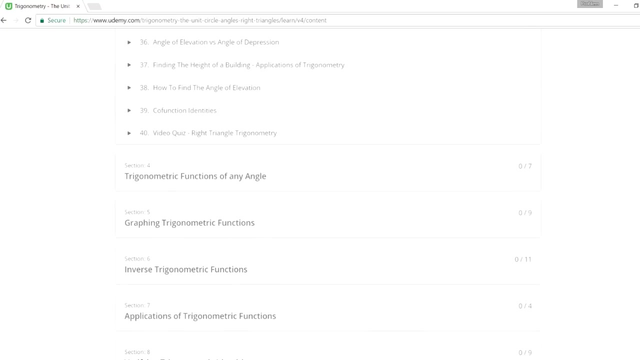 problems, arc length, information on the unit circle, how to evaluate trigonometric functions using the unit circle, right triangle trigonometry, things like SOHCAHTOA. even you can have video quizzes as well, solving word problems like angle of elevation problems. and then you have next section, graphing sine. 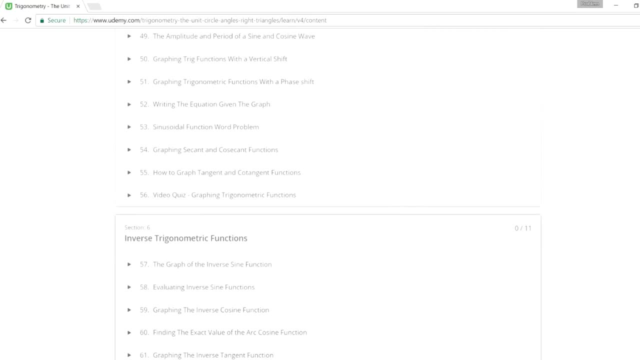 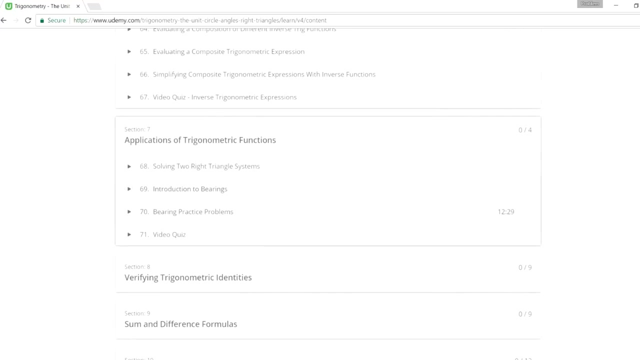 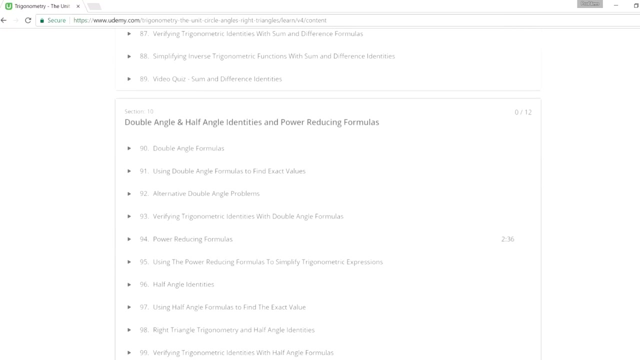 cosine functions, secant tangent, inverse trig functions, pretty much all the common stuff that you'll see in a typical trigonometry course, even solving Barron's verifying trigonometric identities, some indifference formulas, double angle, half angle and some other things too, and, as I mentioned before, I'm gonna add some other things as well. so